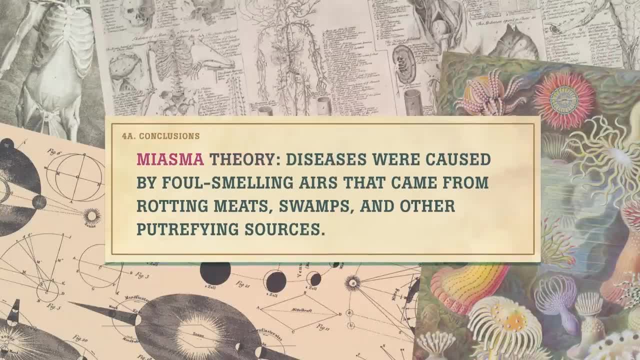 the environment called miasma. According to miasma theory, diseases were caused by foul-smelling airs that came from rotting meats, swamps and other putrefying sources. Before you knock it, think about it. This theory mostly works. Dangerous microbes grow. 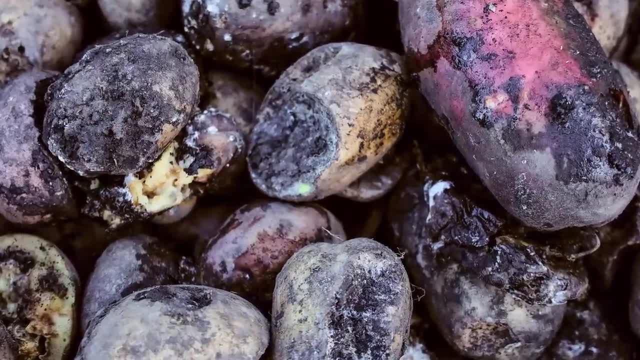 on smelly dirty stuff. The smell is a byproduct of the microbes eating organic matter. But even today we can't see the microbes without it. So why would we want to know how they did it? We can't see microbes without instruments. 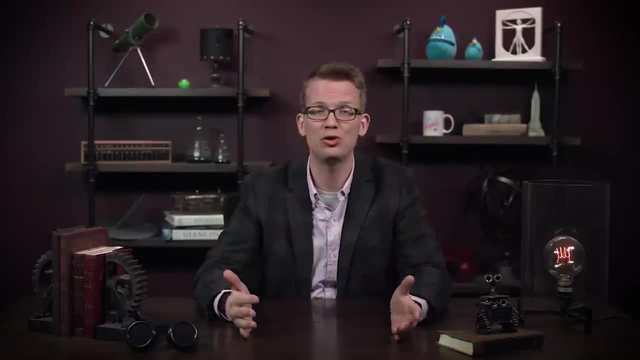 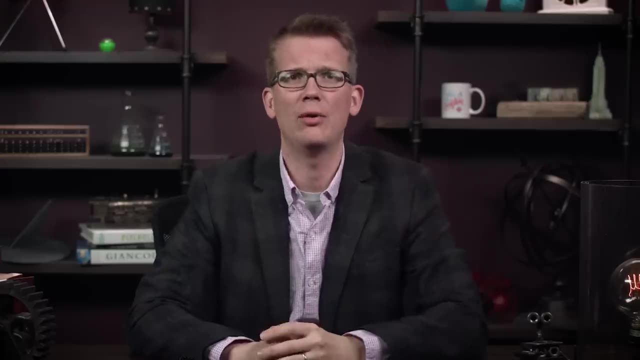 So following our unaided senses is still smart. Don't eat gross trash. Sniff the turkey before you eat it And then just eat it anyway, like I did this morning. By the mid-1800s, however, a few scientific rebels were pushing a germ theory of disease. 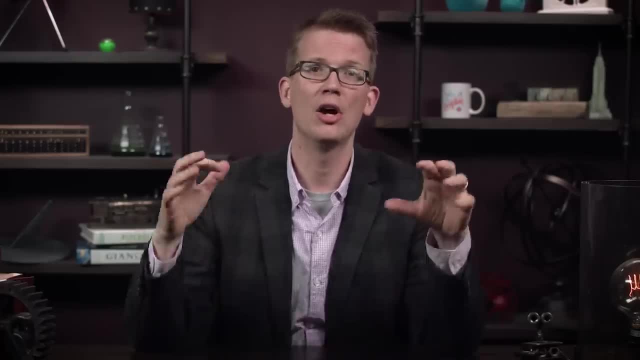 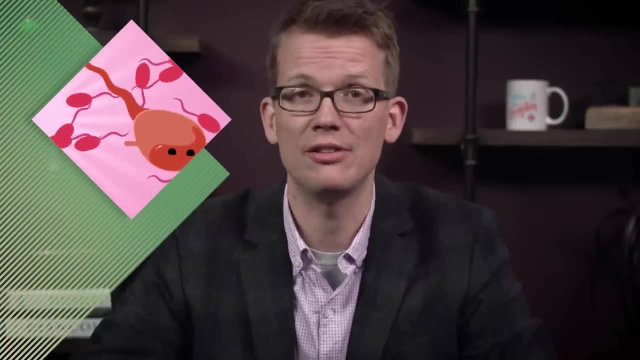 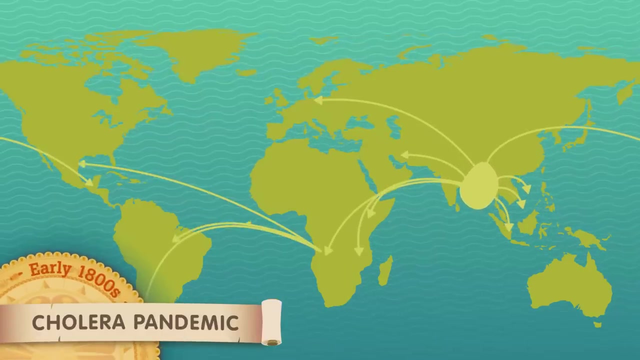 This holds that germs or pathogenic microorganisms cause infectious diseases. Around this time a nasty germ called Vibrio cholerae provided an opportunity to test the theory out. Wow, And since the germ started to travel widely out of South Asia in the early 1800s, hitching. 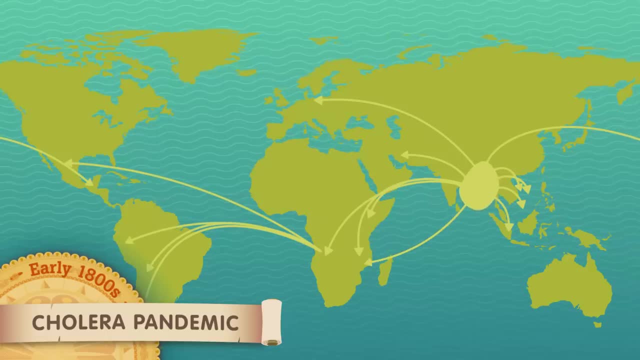 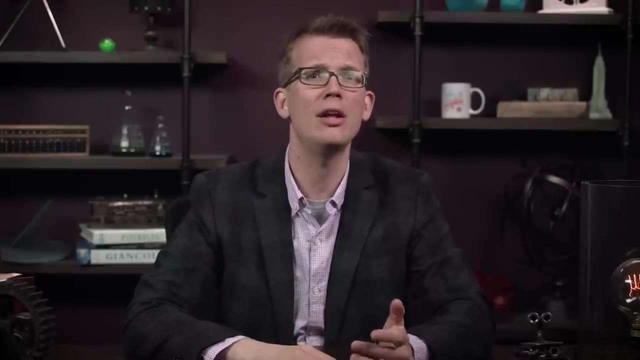 rides on the expanding armada of merchant ships. empire had all kinds of unpredicted downsides. In 1854, a bad cholera epidemic hit Broad Street in the Soho neighborhood of London, killing over 600 people. One doctor named John Snow had a hunch about what was going. 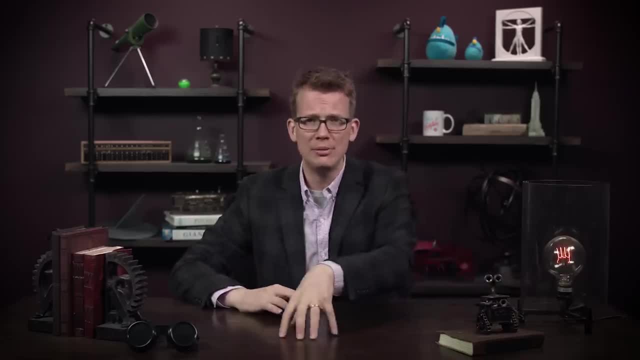 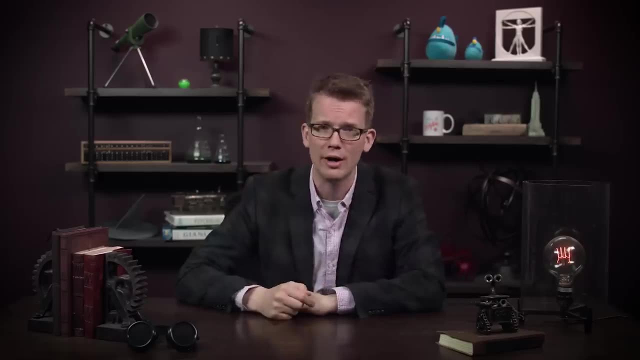 on. Snow created a map of the outbreak and noted that the cases seemed to cluster around one public well. He hypothesized that cholera microbes were rapidly increasing and that they were causing more and more diseases. So he convinced the Soho Council to remove the well's pump handle. People went elsewhere. 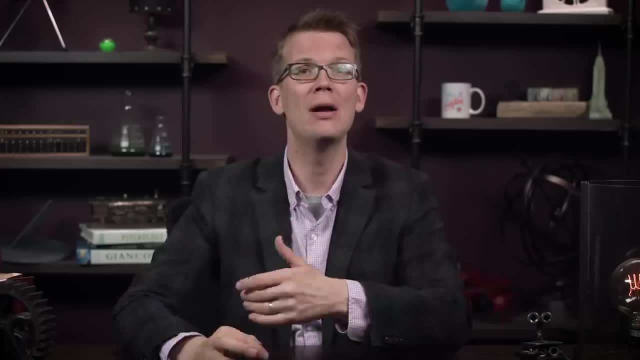 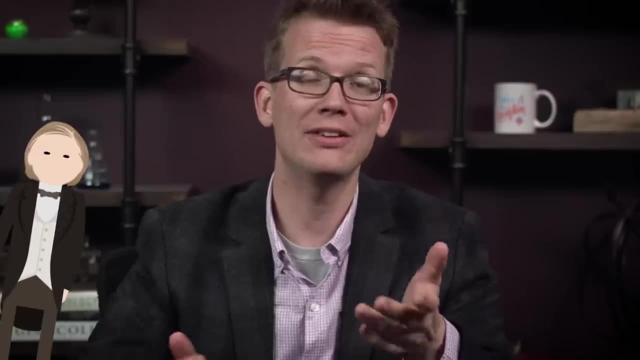 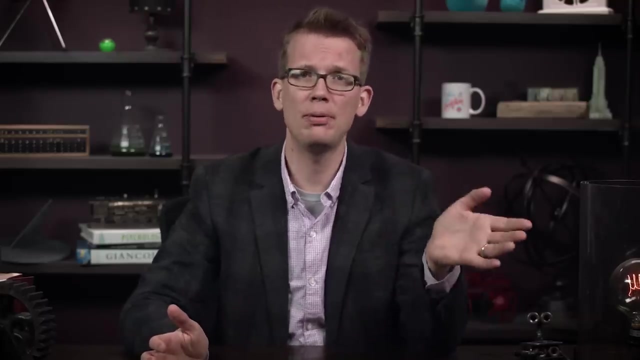 for their water, and cholera infections decreased. John Snow became a hero, saving lives, even though, it turned out, the outbreak was already in decline when he removed the handle, Thus proving that some John Snows do know some things. John Snow's quick thinking didn't really prove germ theory For germs to replace miasmas. 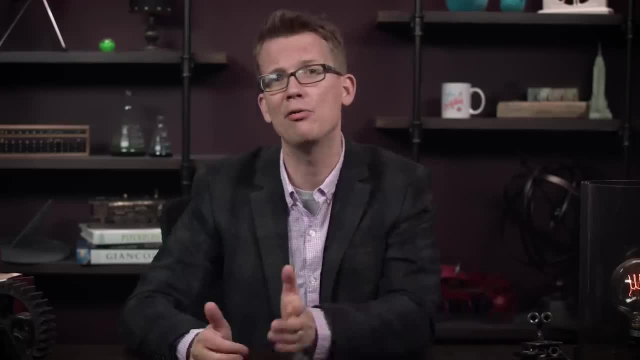 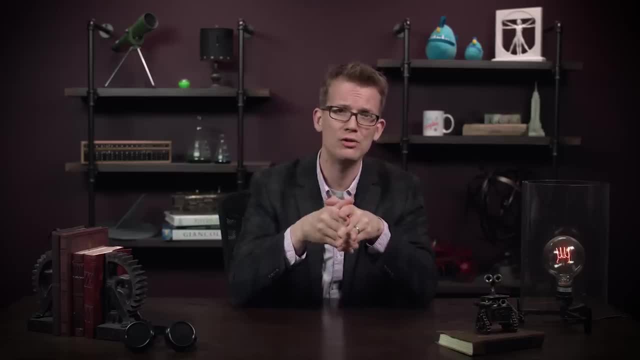 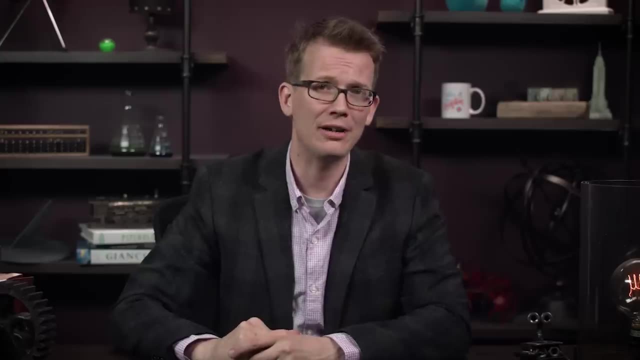 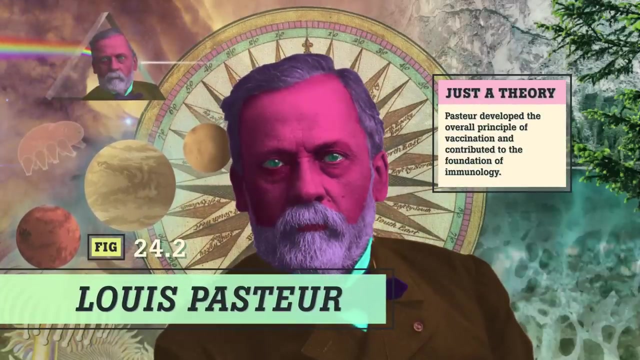 He was right. For that we turn to one of the first experimental microbiologists And a dude whose name you probably should know from milk labels. Louis Pasteur, Born in France in 1822, the same year as Galton, Pasteur, was a chemist, not a physician, But he is known for his work. 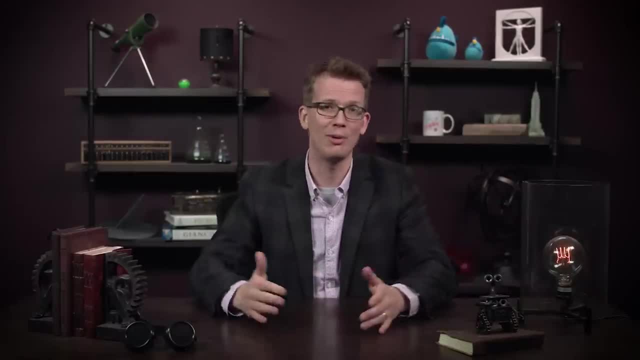 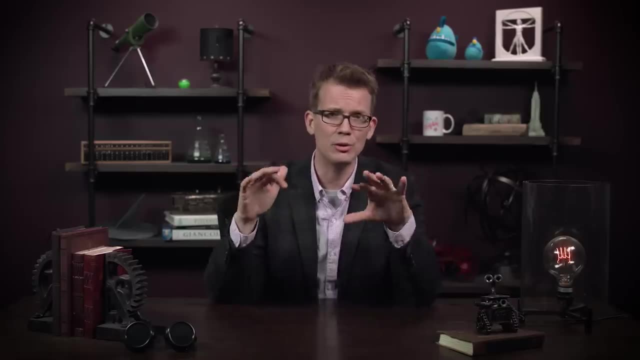 on germs and health. Pasteur is credited as the co-founder of microbiology and the founder of modern zymology, the science of fermentation. Fermentation is the biological and chemical process needed to make beer, wine, yogurt, cheese, bread, lots of other foods. 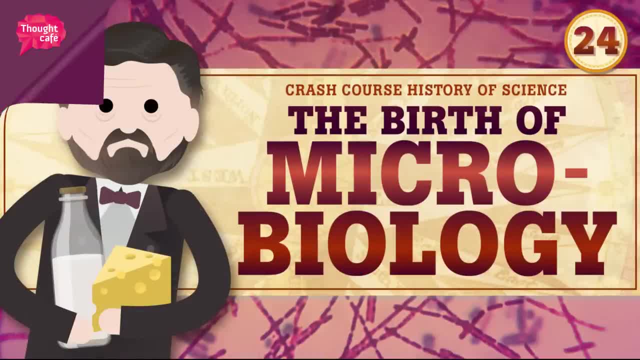 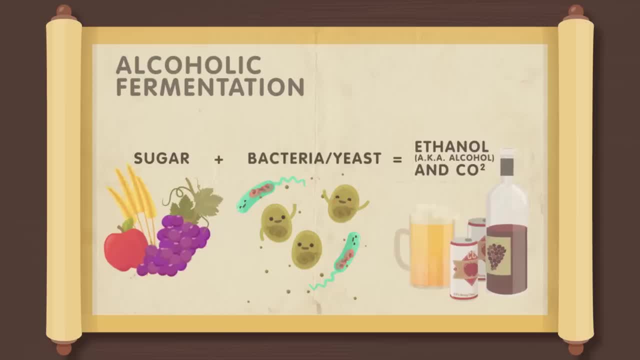 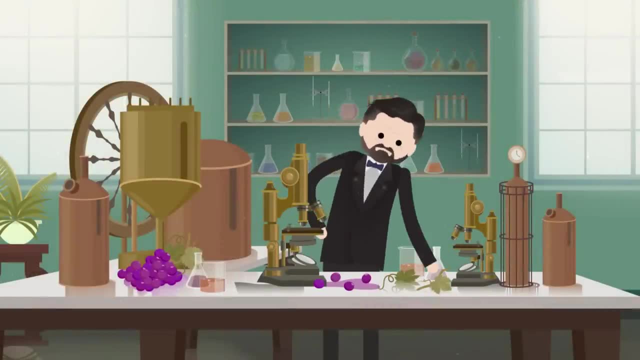 Thought Bubble show us what that means Chemically. fermentation is the conversion of sugar molecules into ethanol or alcohol and carbon dioxide In food. this usually happens thanks to bacteria or yeast Looking good Saccharomyces Pasteur first connected yeast to the fermentation of wine in 1857.. 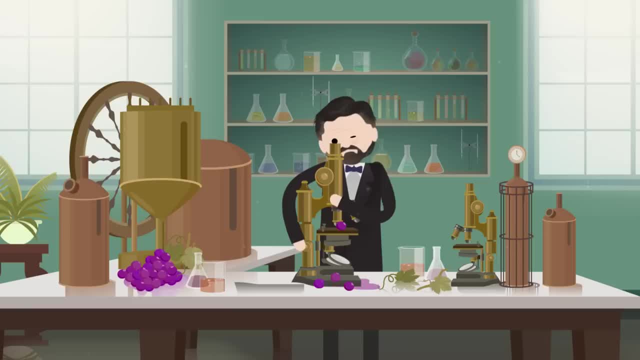 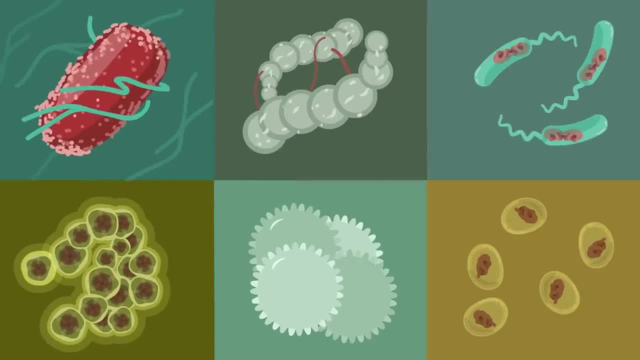 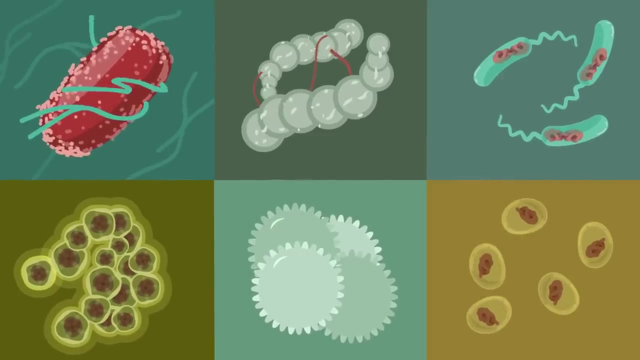 He observed that microscopic yeast on grape skins makes grape juice ferment into wine. If you sterilize the skins, killing the yeast, fermentation won't happen. Pasteur even made the analogy that the microbes growing in wine and beer were similar to the microbes causing diseases in humans and animals. 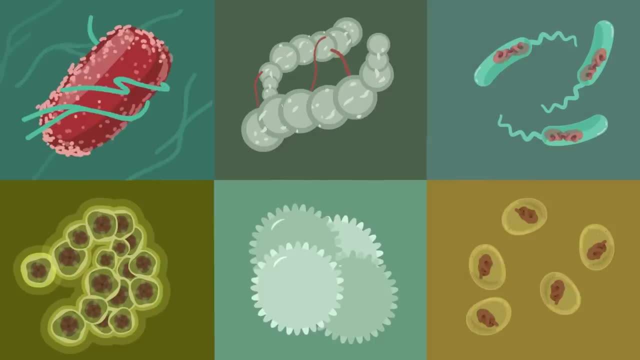 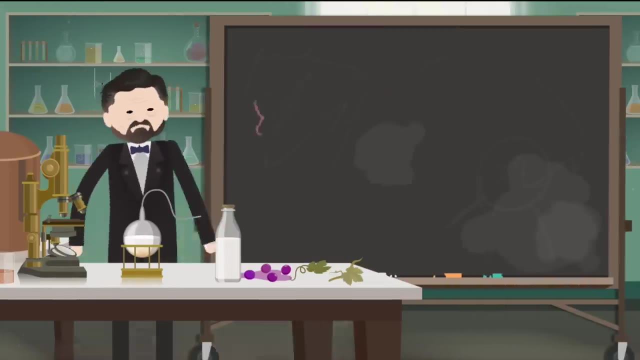 He hypothesized that microbes are everywhere and must be responsible for all kinds of phenomena, like making food spoil. So in 1865, he patented a process in which liquids such as milk were heated to a temperature between 60 and 100 degrees Celsius in order to kill microbes. 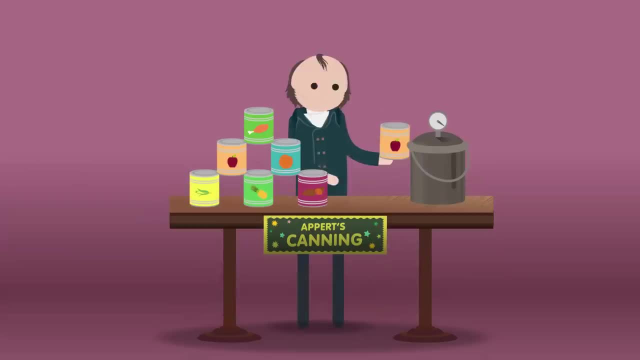 This became known as pasteurization. This might sound kind of simple, but it was revolutionary. Earlier Nicolas Appert had invented canning to make food safe, so Napoleon could fight wars for longer. But Pasteur's method used a lower temperature, thus preserving tastes and textures. 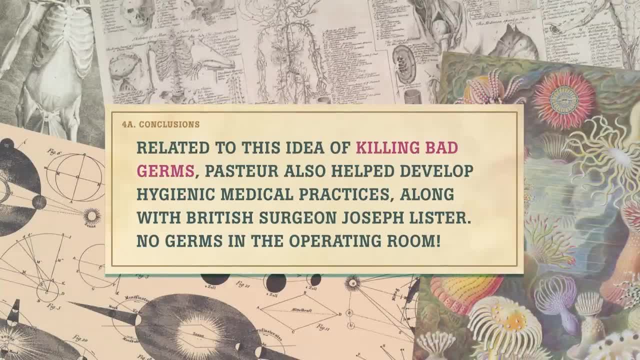 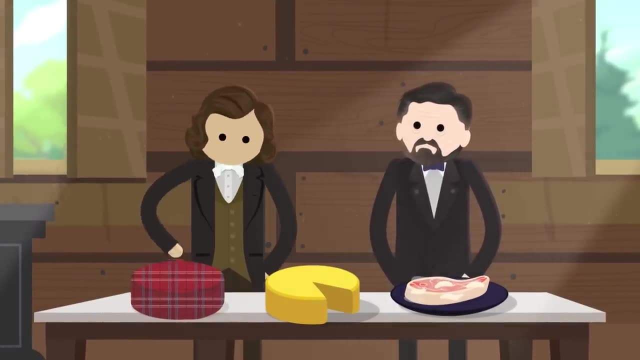 Related to this idea of killing bad germs, Pasteur also helped develop hygienic medical practices along with a British surgeon, Joseph Lister. No germs in the operating room. Most importantly for the history of biology, Pasteur got tangled up in a debate with a fellow scientist named Félix Pouchet, who 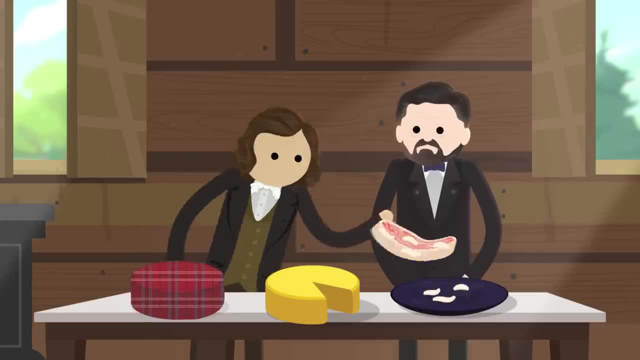 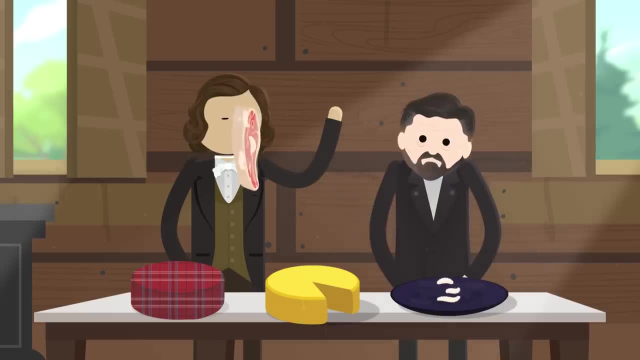 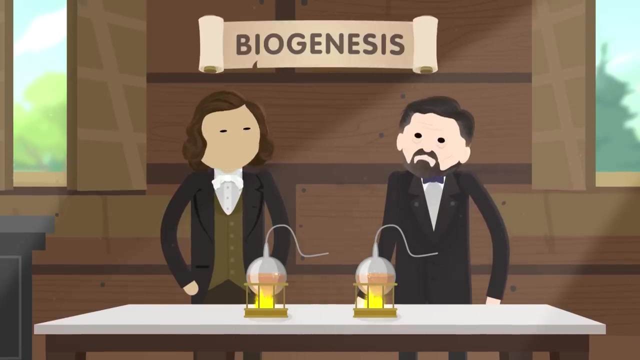 believed that living things spawn naturally from certain environments. This widely-held belief was called spontaneous generation. Pasteur, based on his observations of grapes, reasoned that living things can only grow from other living things. So he created an ingenious experiment to prove the theory of biogenesis, or life from life. 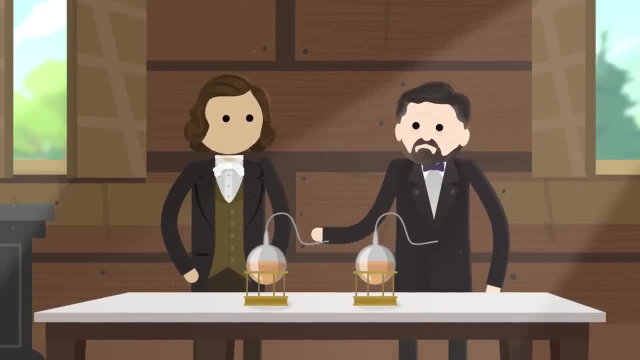 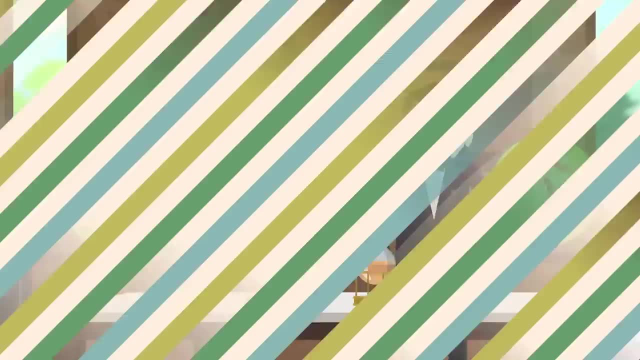 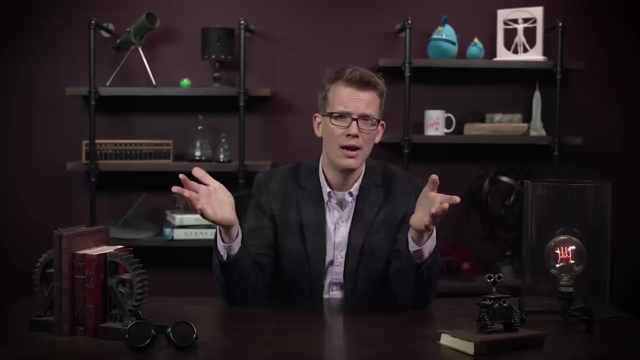 Pasteur showed that no germs would grow in sealed, sterilized long-necked fruits, But in sterilized but open flasks microbes would eventually show up. Thanks Thought Bubble. After proving biogenesis in the 1870s, Pasteur worked on immunology and vaccination. 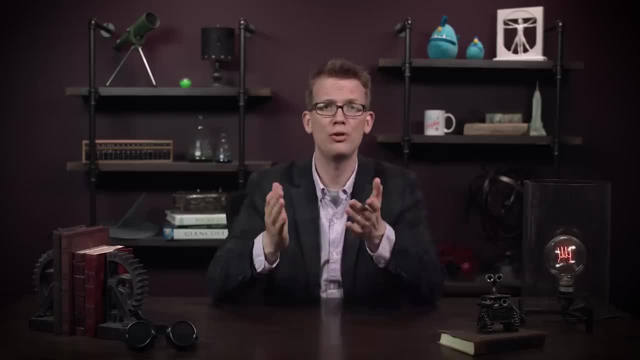 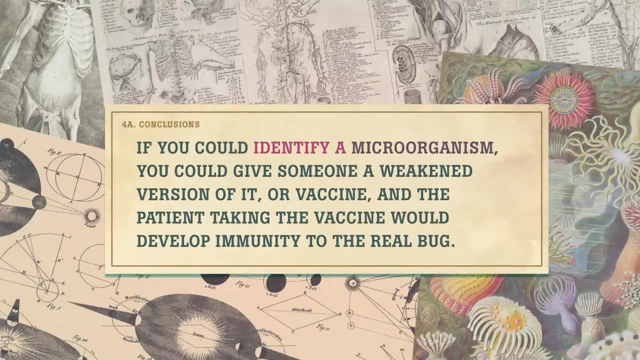 Pasteur's work with the rabies and anthrax microbes supported the germ theory and its use in medicine. If you could identify a microorganism, you could give someone a weakened version of it or vaccine, and the patient taking the vaccine would develop immunity to the real bug. 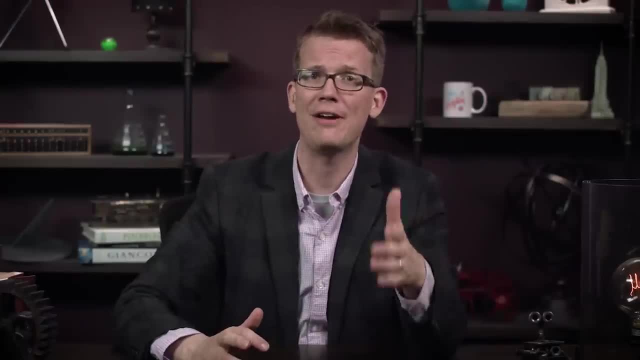 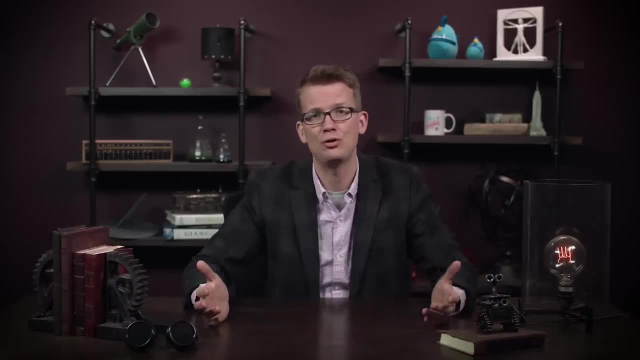 And in 1879, Pasteur was able to do that. In 1879, Pasteur developed the first lab-manufactured vaccine for chicken cholera. It was about this time that germ theory was finally widely accepted, in part due to Pasteur's 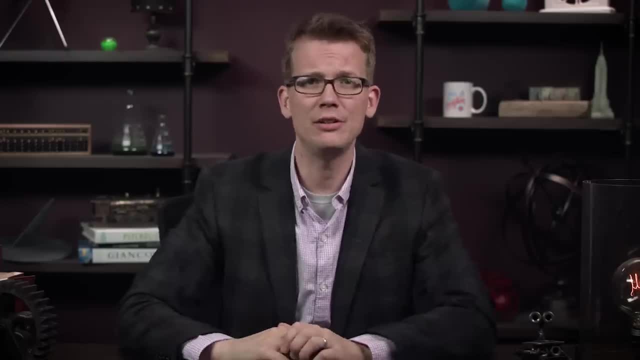 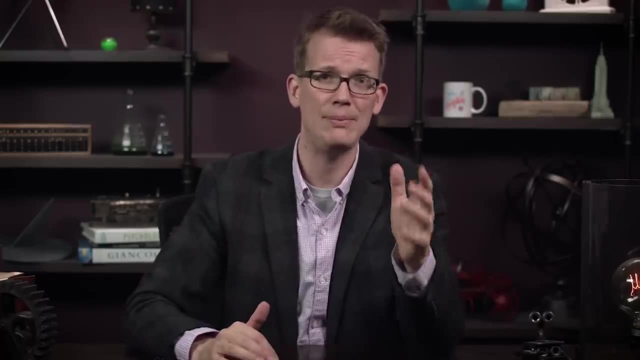 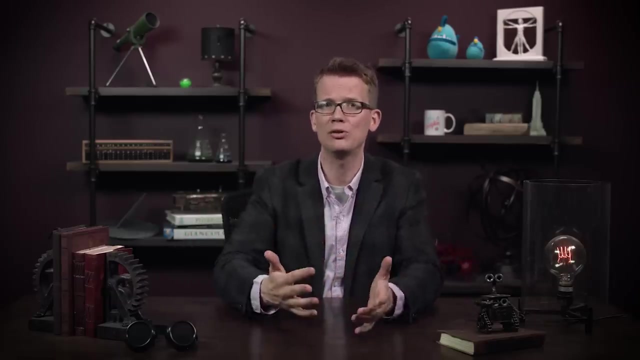 work, But Pasteur's ethics were questionable. When rabies vaccines for humans rolled out, Pasteur kept his data on their effectiveness secret. He even kept secret mortality data, or how many people his vaccines didn't help. So, unlike today, in Pasteur's time it wasn't necessarily a norm that useful medical research. 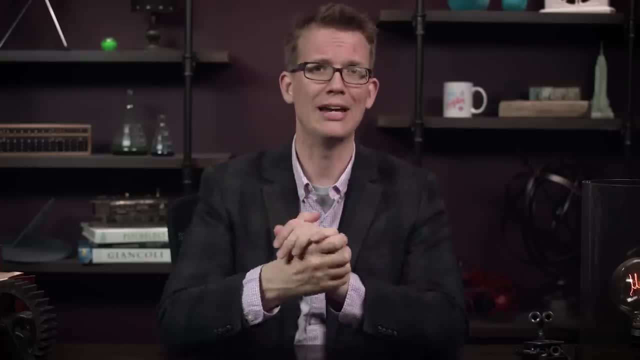 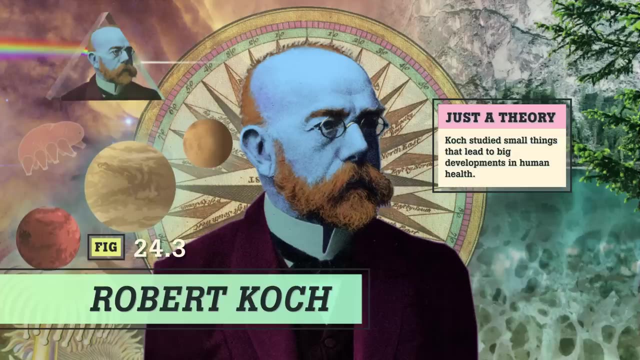 should be shared publicly. But Pasteur was not the only one. Pasteur was the only notable germ wrangler Born in 1843, the German physician Robert Koch painstakingly worked at a microscope to definitively establish the germ concept of disease. 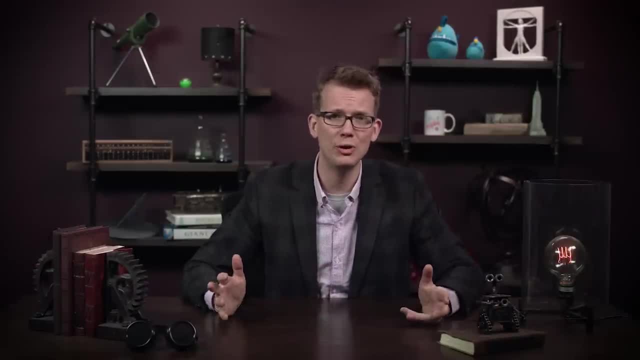 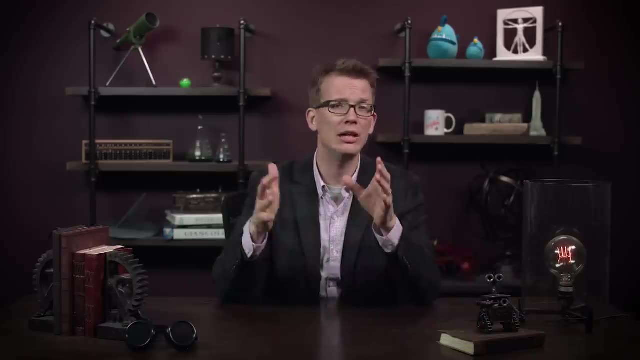 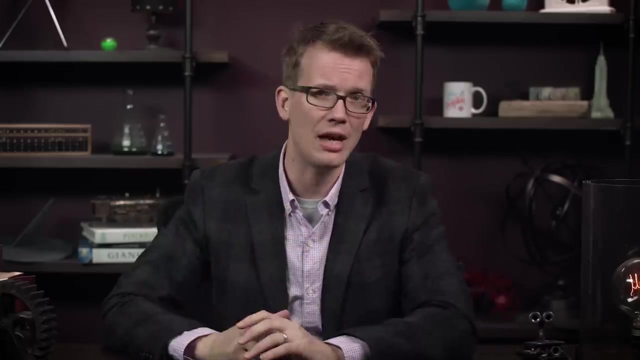 He identified different microbes, becoming the leader of a large research team in Berlin. They founded the Discipline of Bacteriology, or the Study of Bacteria, particularly in relation to human health. In the late 1880s and 90s, Koch and his team traveled into areas experiencing epidemics. 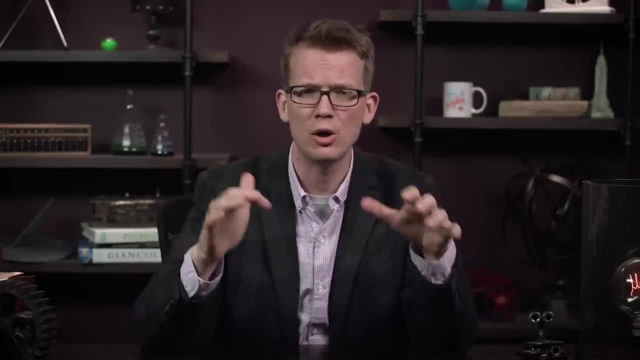 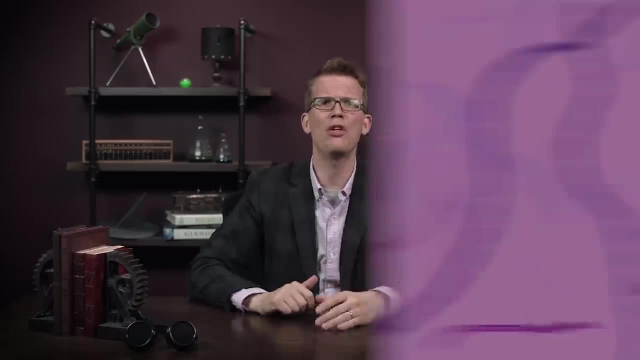 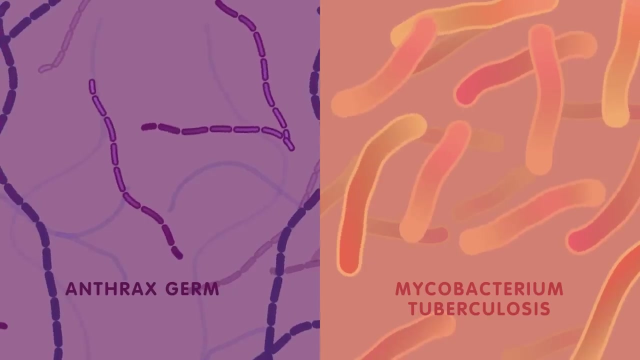 including India and India. They were able to identify the microbes causing the diseases there. By ID'ing these microorganisms, they hoped to create vaccines. First, Koch proved that the anthrax germ causes anthrax the disease. Later he identified the bacterium that causes tuberculosis or TB, which was a very widespread 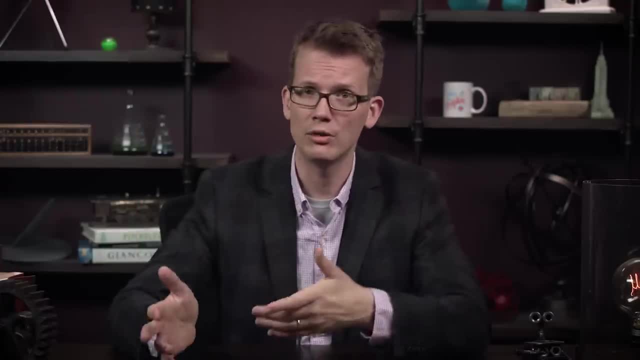 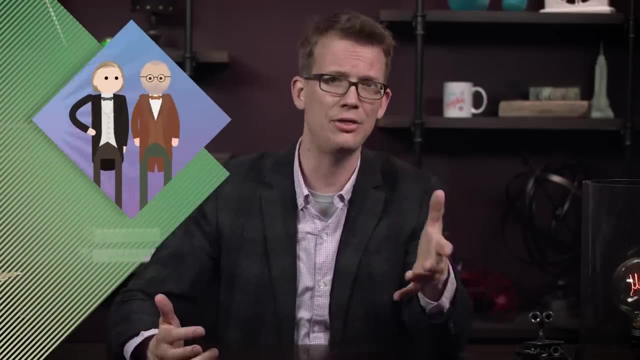 disease. Koch also characterized cholera, vindicating the work of John Snow by showing that the bacterium lives naturally in the small intestine of humans. Snow wasn't just high on ether. He had correctly guessed that. He had perfectly guessed how cholera spreads. 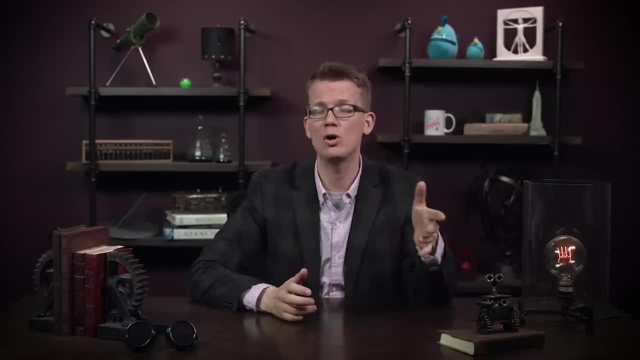 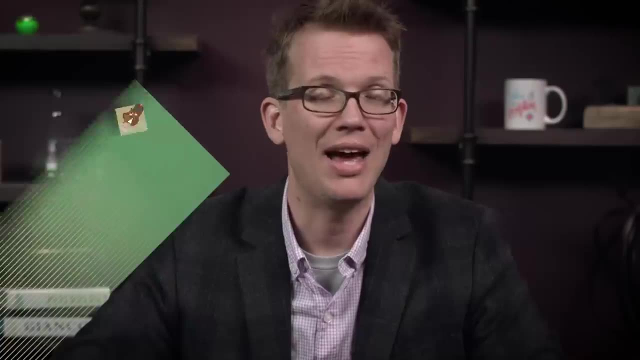 Eventually, Koch's team contributed to the identification of the germs that cause diphtheria, typhoid, pneumonia, gonorrhea, meningitis, whooping cough, tetanus plague, leprosy and syphilis. 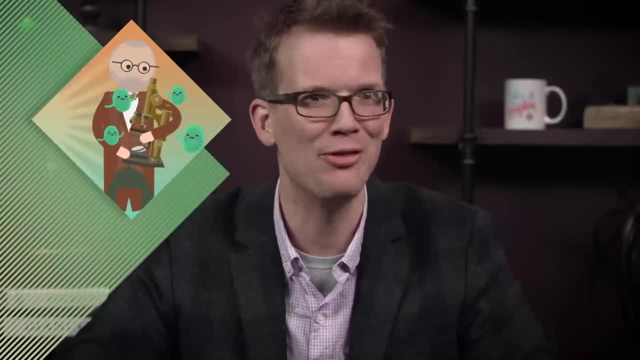 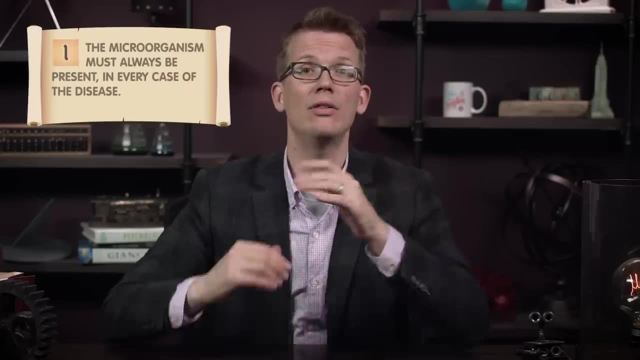 I wouldn't want to borrow this dude's lucky microscope. It's been through a lot. Through this work, Koch developed the four postulates or steps for identifying infectious diseases. 1. The microorganism must always be present in every case of the disease. 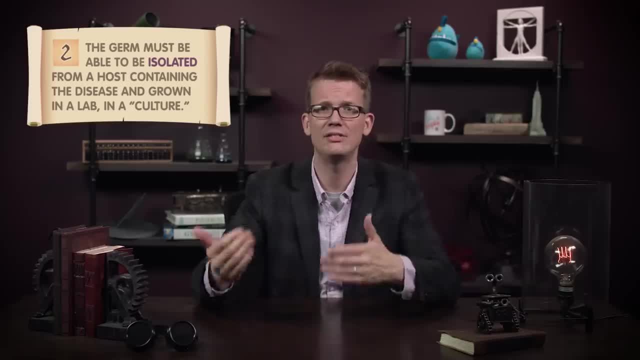 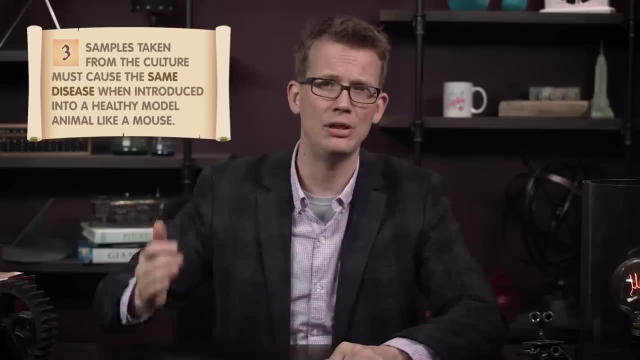 2. It must be able to be isolated from a host containing the disease and grown in a lab in a culture. 3. Samples taken from the culture must cause the same disease when introduced into a healthy model animal like a mouse. 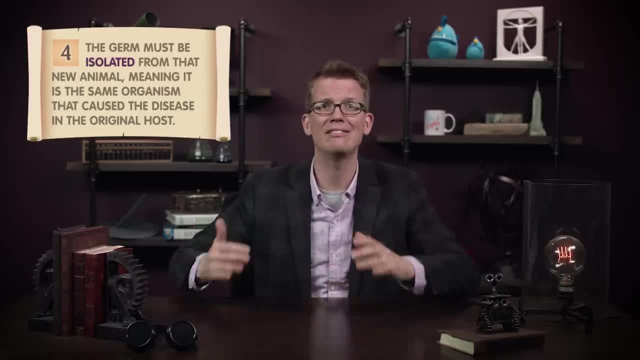 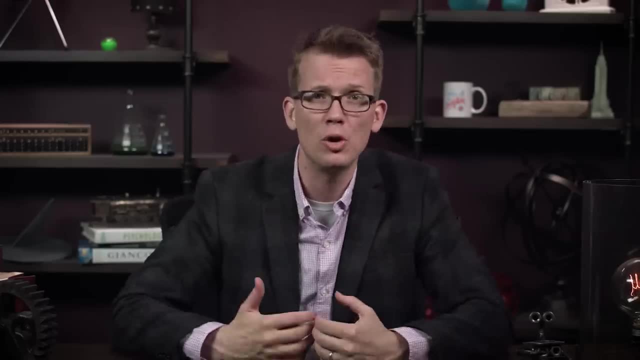 4. The germ must be isolated from that new animal, meaning it's the same organism that caused the disease in the original host. So structure matters In all infections. germs grow out of hand, throwing the body out of whack and causing 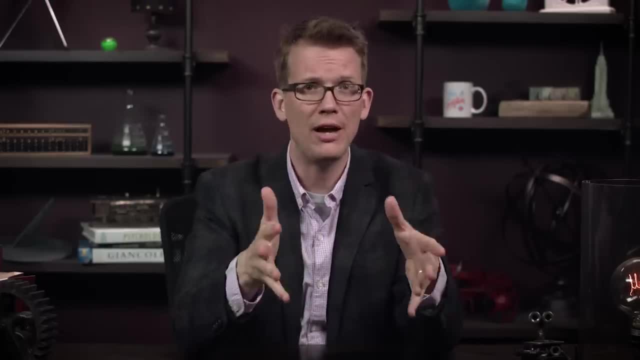 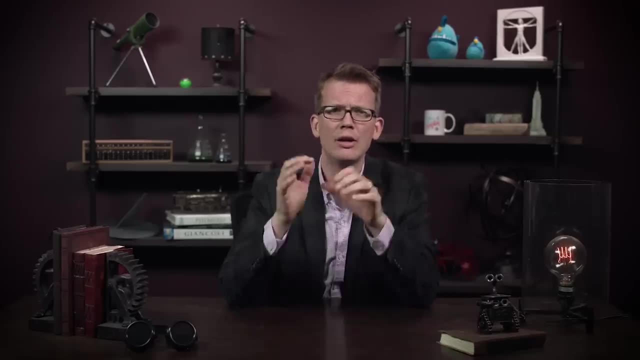 inflammation. 5. All germs or pathogens develop and live within us and can kill us, But with Pasteur's vaccines and Koch's scientific method of IDing bacteria, humans could now develop medicines to fight jerk-sauce germs. 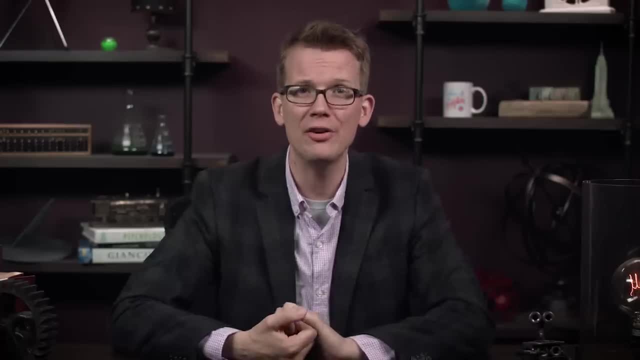 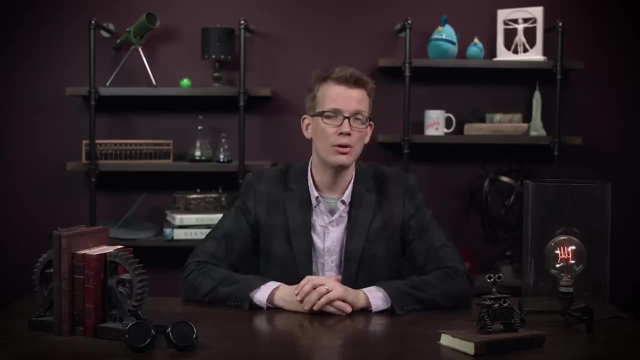 Go, team us Back in the world of multicellular organisms. another scientist, at the intersection of biology and medicine, was exploring the structure of living things. In 1892, German-American physiologist, Jacques Loeb, began experiments on embryonic development, or how organisms grow from the body. 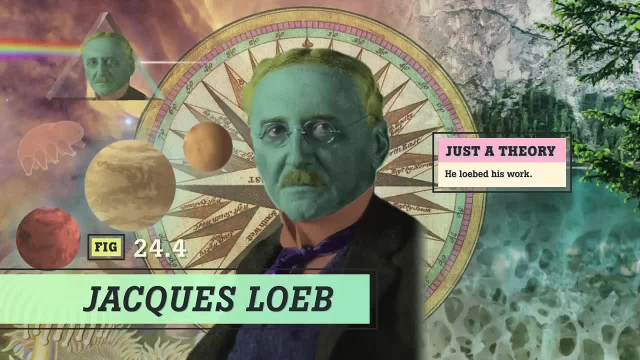 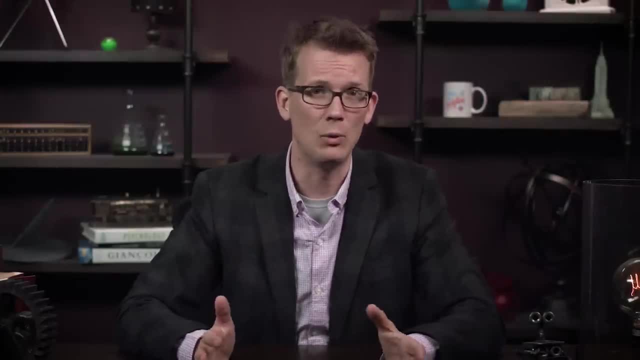 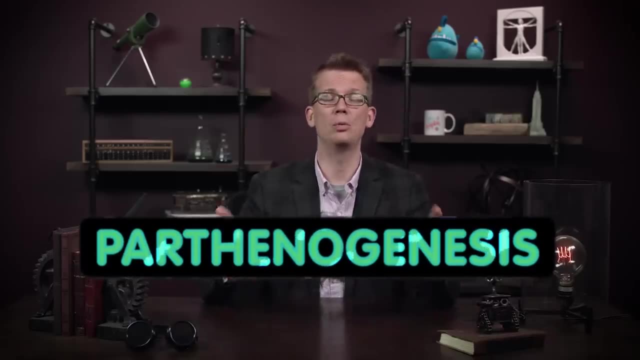 He started dunking sea urchin embryos into different salt solutions and in 1899 he got one to give birth just from being salty. Loeb's artificial parthenogenesis, or birth from the self, was mega-astounding news. 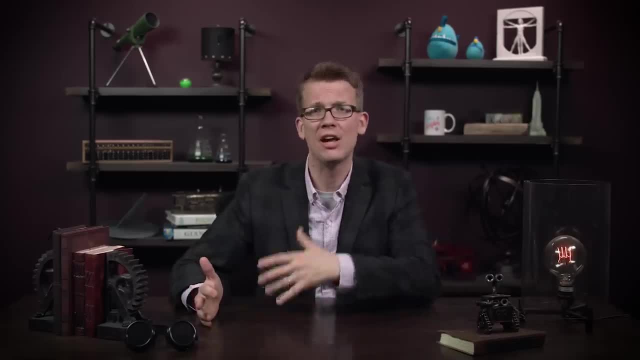 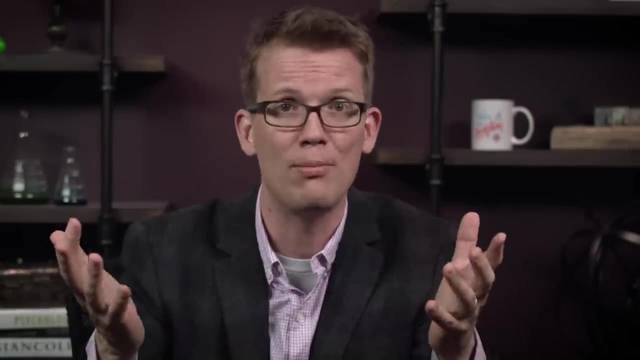 It raised basic questions like: what is sex? Could a human one day give birth by herself or himself? Causing sea urchins to give virgin births Made Loeb a celebrity, But for the history of biology it was revolutionary that Loeb's sense of scientific understanding. 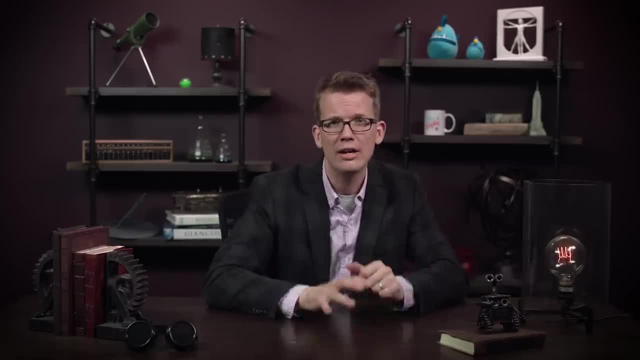 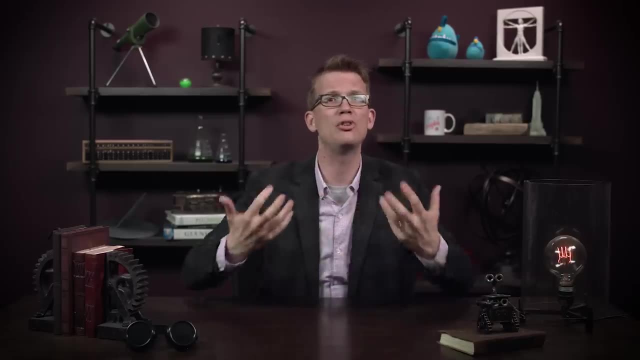 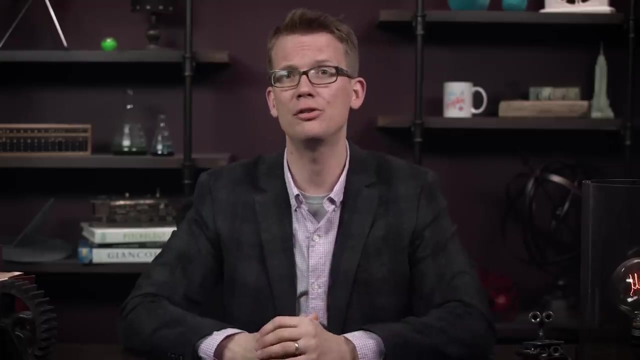 of life was tied to his ability to control it. His work with sea urchins can be seen as an early form of bioengineering, or treating cells and tissues as machine parts to be used constructively by a human designer. Loeb's notable students included the behavioral psychologists B F Skinner and J B Watson.